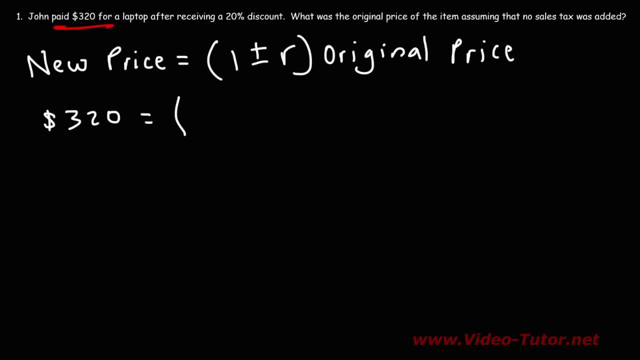 price. So that's why we need to use negative r instead. If the percentage were to increase the price like a sales tax, we would use positive r. So since we're dealing with a discount, it's going to be 1 minus r. Now what is r? R is 20%, But you don't want to plug it in as a percentage. You want to. 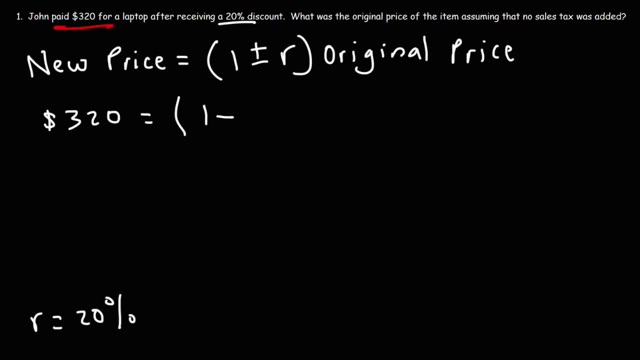 plug it in as a decimal, So you need to know how to convert a percent into a decimal. Well, there's two things you can do. You could divide 20% by 100%. You could divide 20% by 100%. You could divide. 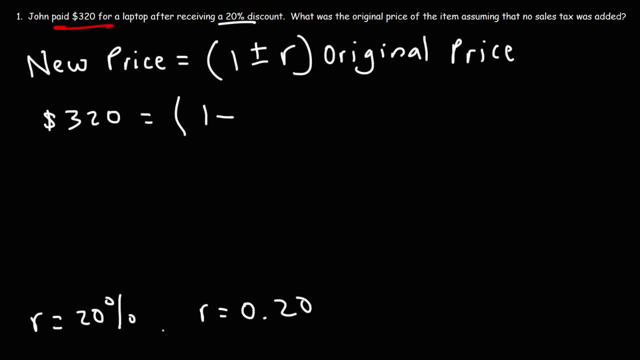 20% by 100%, And that will give you 0.20.. Or you could simply move the decimal two units to the left, which will still give you 0.20.. So that's our r value, The original price. we don't know what. 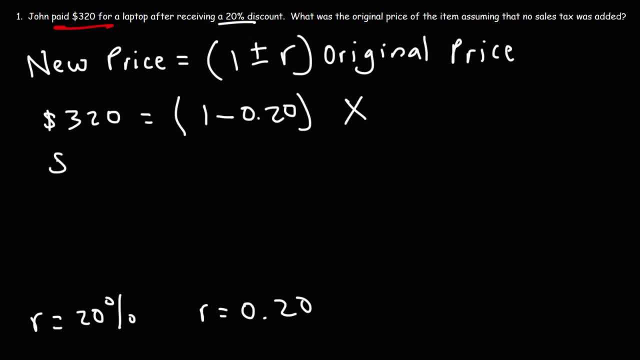 it is, So we're going to call it x. So 1 minus 0.20 is 0.80.. So what this means is that, after receiving a 20% discount, the new price is 80%. Now, in order to calculate the original price, we need to divide both sides by 0.80.. So the answer? 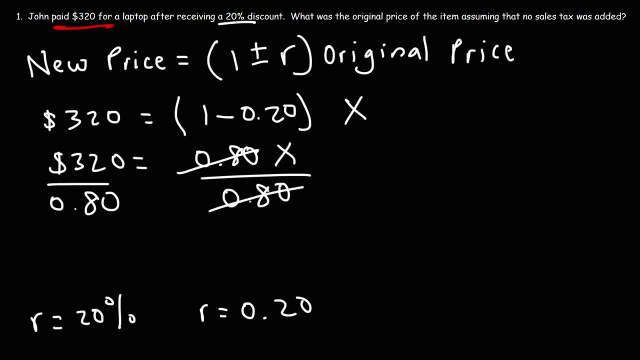 is going to be 320 divided by 0.80.. Thus the original price of the laptop was $400.. After he received a 20% discount it went down to 320.. And you could check your answer. You could find out. hey, what is 20% discount And you could check your answer. You could find out, hey, what is 20% discount And you could check your answer. You could find out, hey, what is 20% discount. 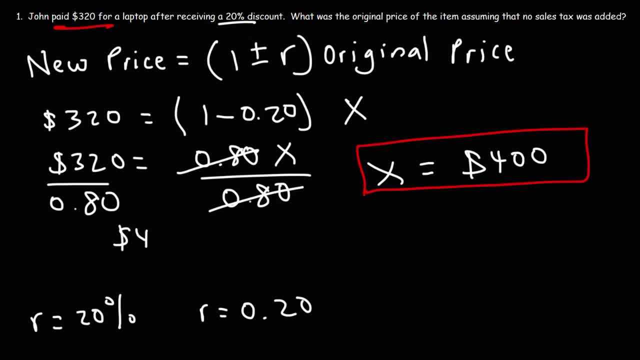 20% of 400.. 10% of 400 is $40.. You just need to move the decimal one unit to the left. So 20% of 400 is twice the value of 10%, which is 40.. Twice the value of 40 is 80.. So that's 20% of 400. 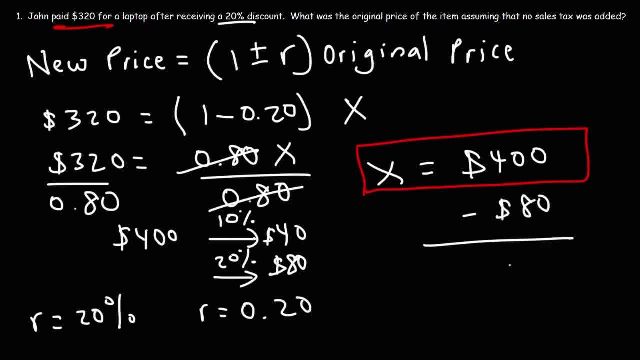 So if you take off $80,, this will give you the new price of the laptop after the discount, which is 320.. And so that's a quick way that we could use to check our work. But the final answer for this problem.